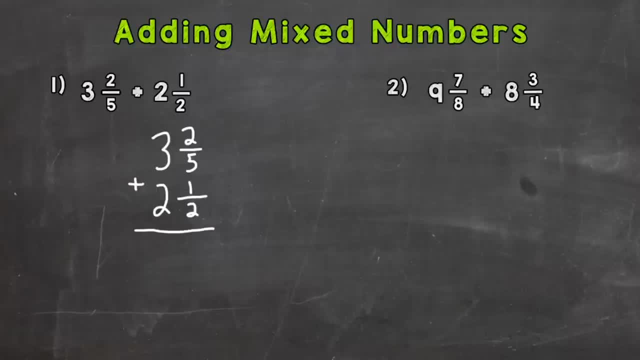 fractions are lined up and my whole numbers are lined up Now, just like when we add fractions that don't have the whole number involved, we need a common denominator. So we still need a common denominator for these problems. if we don't have one- and obviously we have a five and a two, so we don't have- 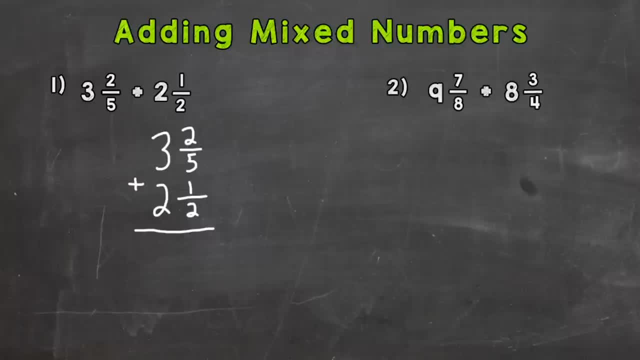 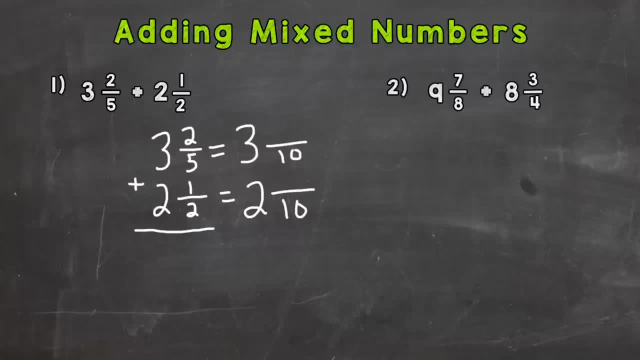 five and a two. So I need to rename two, two, five and a two. I need to rename five, and then I need to rename the top part with the original denominator, But the rest are mit Fellet Brooklyn over here. Let's go to that. 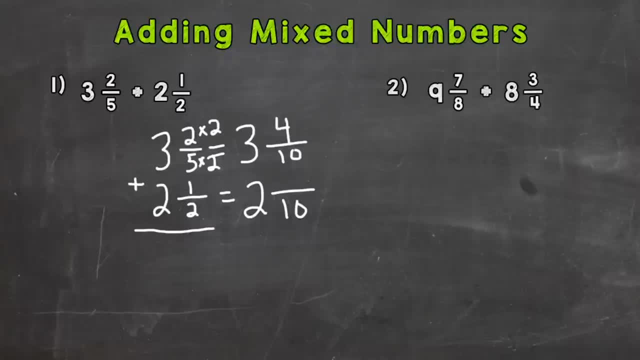 and let's remind our раздел and start looking like two times four respectively: goddess and budget four. Guys, you can't do that without some common denominator in here. so there you go frnisly, a common denominator of 10.. So let's do the second one. 2 times 5 gives me that. 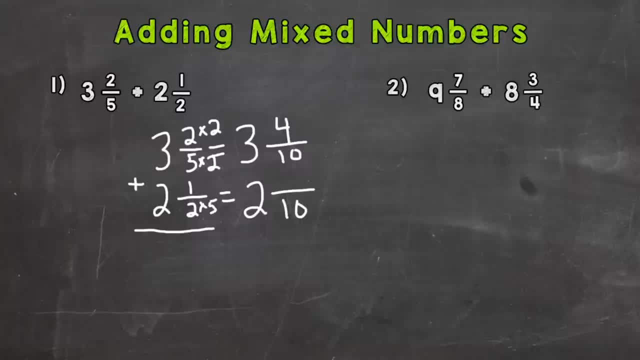 common denominator of 10, so I need to do the same thing to the top in order to get an equivalent fraction. 1 times 5 is 5. And if you think about it, a half is the same as 5 out of 10.. Again, we didn't change the value of the problem Now that 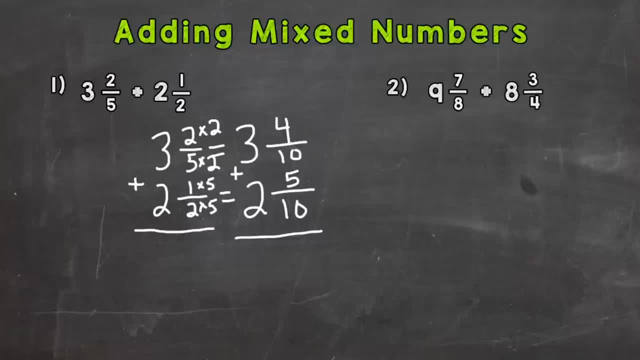 we have a common denominator we can add. So 4 plus 5 gives me 9.. Keep our common denominator of 10 the same. So 9 tenths is going to be our fractional part. Now we need to do the whole numbers. 3 plus 2 is 5.. Now you always check to see if the 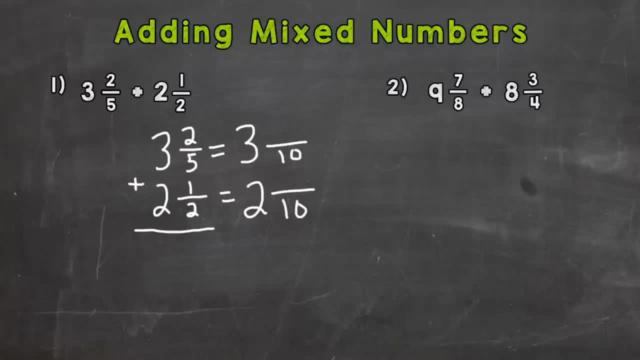 rename both of these mixed numbers, the fractional part, with the common denominator of 10.. So I've got to think to myself here: 5 times 2 is 10, so I need to do that same thing to the numerator or top in order to find an equivalent fraction here. 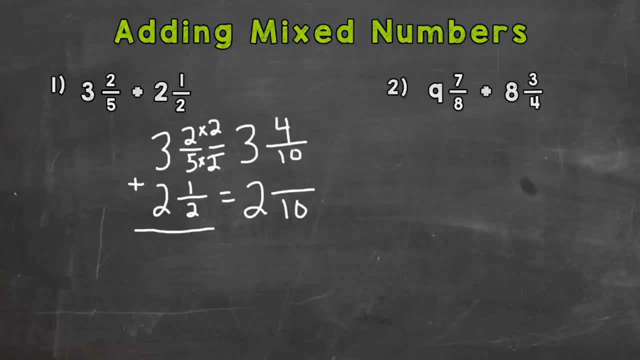 So 2 times 2 is 4.. I'm not changing the value of the problem, I'm just renaming with a different denominator So they both have a common denominator of 10.. So let's do the second one. 2 times 5 gives me that common denominator of 10,. 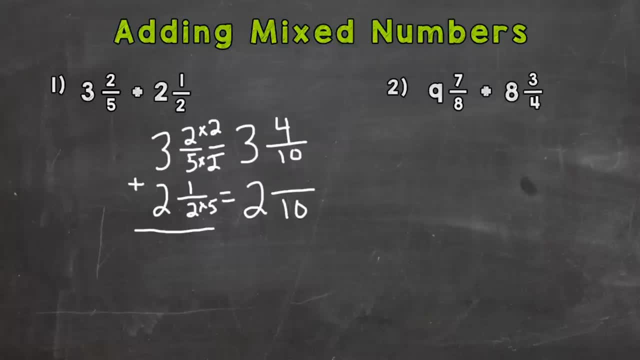 so I need to do the same thing to the top in order to get an equivalent fraction. 1 times 5 is 5. And if you think about it, a half is the same as 5 out of 10.. Again, we didn't change the value of the problem. 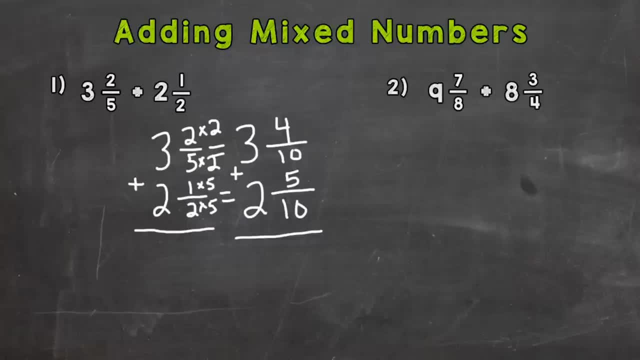 Now that we have a common denominator, we can add: So 4 plus 5 gives me 9.. Keep our common denominator of 10 the same. So 9 tenths is going to be our fractional part. Now we need to do the whole numbers. 3 plus 2 is 5.. 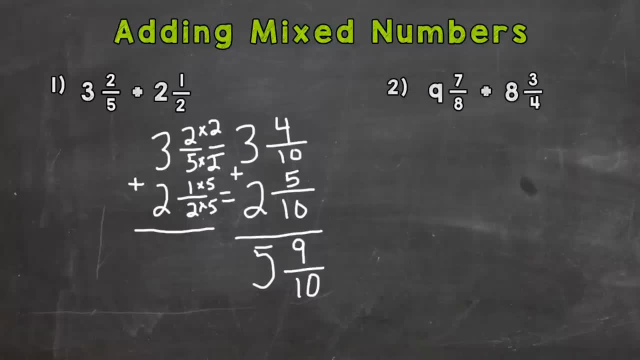 Now you always check to see if the fractional part can be simplified, and in this case it cannot. So our final answer is 5 and 9 tenths. So let's jump into number 2. here We have 9 and 7 eighths, plus 8 and 3 fourths. 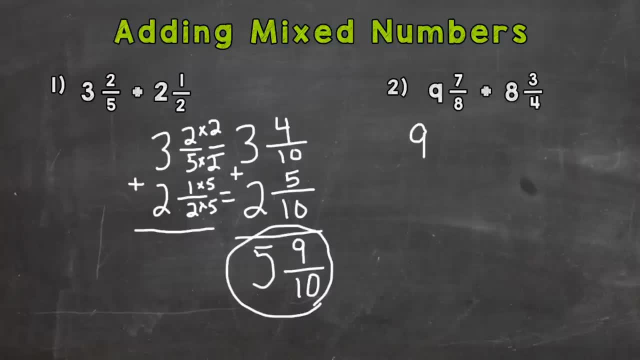 So I'm going to line up my problem: 9 and 7 eighths plus 8 and 3 fourths. So let's take a look at our fractional part. We do not have a common denominator, so we're going to need to rename with a common denominator. 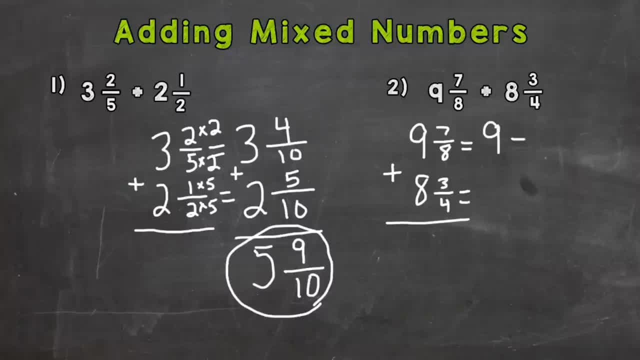 So let's think What's going to be a common denominator for an 8 and a 4?? Well, the common denominator is going to be 8.. So our first fraction, 9 and 7 eighths, already has a denominator of 8.. 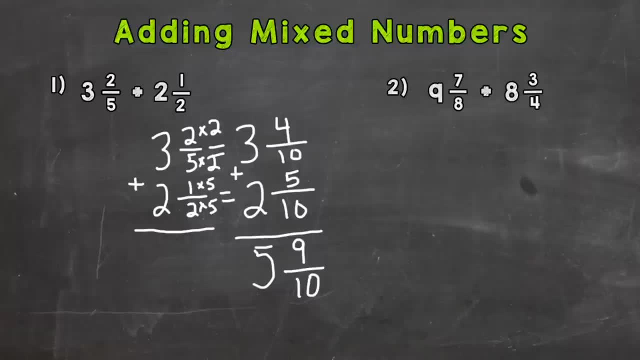 fractional part can be simplified, and in this case it cannot. So our final answer is 5 and 9 tenths. So let's jump into number 2. here We have 9 and 7 eighths plus 8 and 3 fourths. So I'm 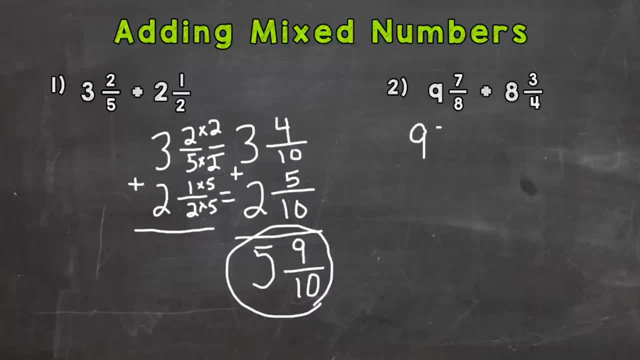 going to line up my problem: 9 and 7 eighths plus 8 and 3 fourths. So let's take a look at our fractional part. We do not have a common denominator, so we're going to need to rename with a common denominator. 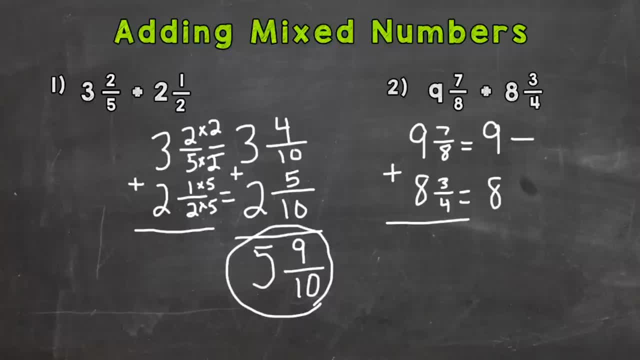 So let's think What's going to be a common denominator for an 8 and a 4? Well, the common denominator is going to be 8.. So our first fraction- 9 and 7 eighths- already has a denominator. 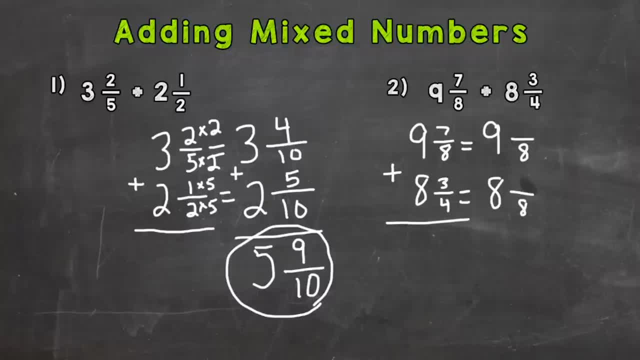 of 8. So we do not need to rename or change that fraction at all. So we're just going to transfer the 7 eighths over. Now we need to rename And we know, 4 times 2 gives us the denominator of 8.. So we need. 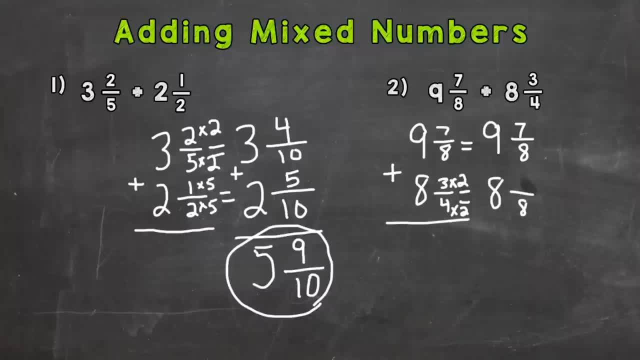 to do the same thing to the top. 3 times 2 is 6.. So 3 fourths is the same as 6 eighths. They hold the same value. We just renamed it so it had a denominator of 8.. 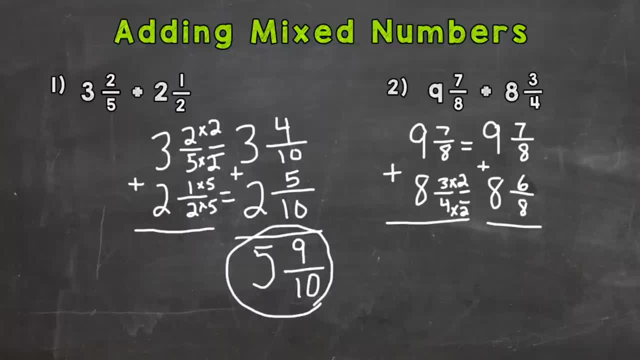 Now we're ready to add, because the fractional parts have a common denominator: 7 plus 6 is 13.. Keep the denominator of 8.. 9 plus 8 is 17.. So our answer is 17 and 13 eighths. Well, our fractional part is an improper fraction. 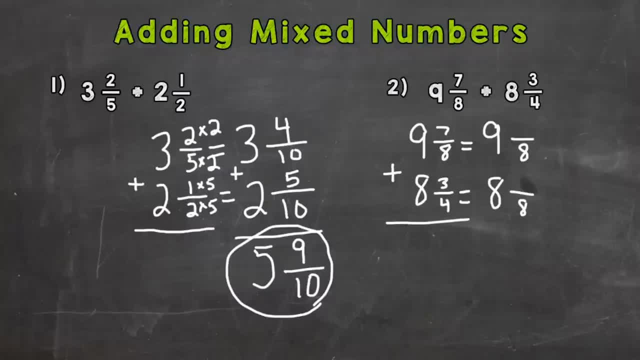 So we do not need to rename or change that fraction at all. So we're just going to transfer the 7 eighths over. Now 3 fourths We're going to need to rename And we know, 4 times 2 gives us the denominator of 8.. 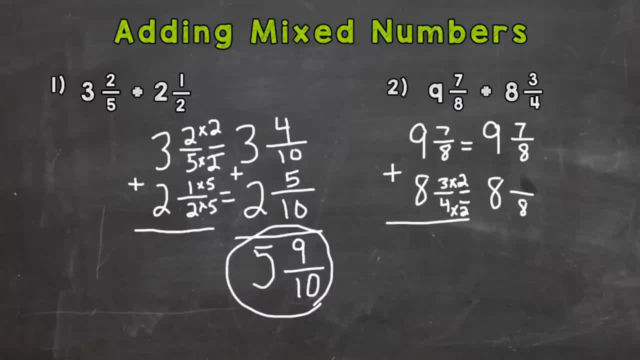 So we need to do the same thing to the top. 3 times 2 is 6.. So 3 fourths is the same as 6 eighths. They hold the same value. We just renamed it so it had a denominator of 8.. 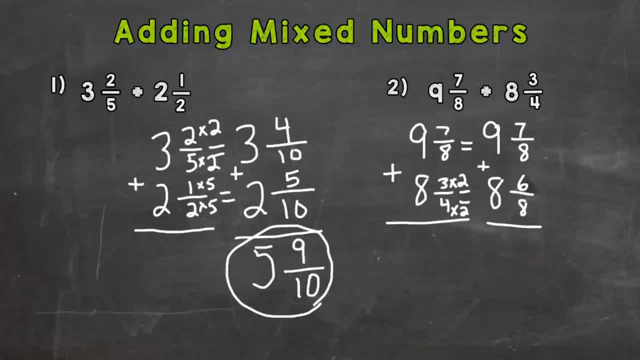 Now we're ready to add, because the fractional parts have a common denominator: 7 plus 6 is 13.. Keep the denominator of 8.. 9 plus 8 is 17.. So our answer is 17 and 13 eighths. 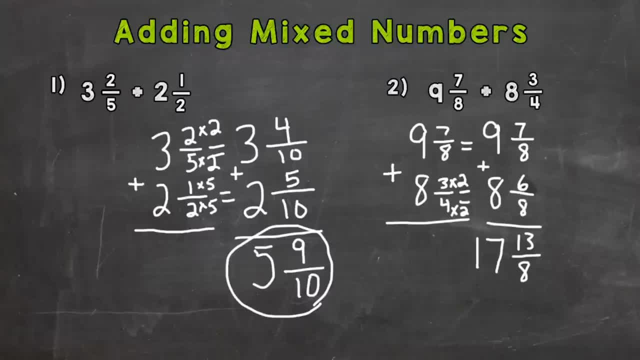 Well, our fractional part is an improper fraction, so we don't want to leave it like that. It's more than one whole, So we're going to change it to the mixed number and we need to combine the whole numbers together. So that's 17 plus whatever whole number we get out of that number. 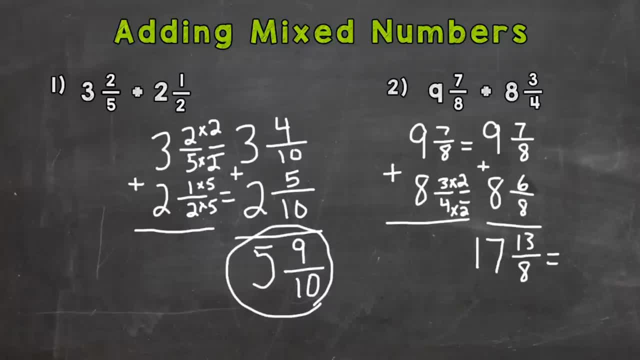 And we're going to get it out of that improper fraction. So we can think of it like this: 17 plus. well, to get improper to mixed number, we need to do the top divided by the bottom, 13 divided by 8.. 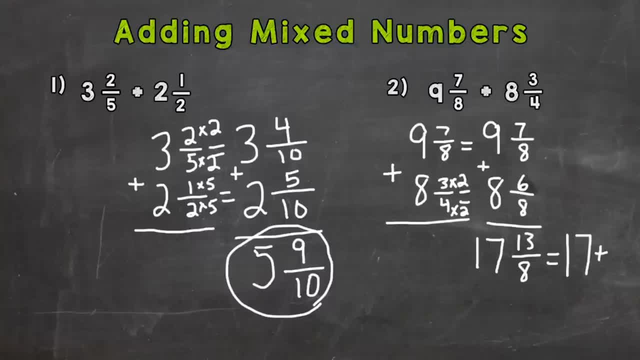 How many whole groups of 8 can we pull out of 13?? Well, one whole group with a remainder of 5.. 5 left over. Keep our denominator of 8 the same, So 13 eighths equals 1 eighths. 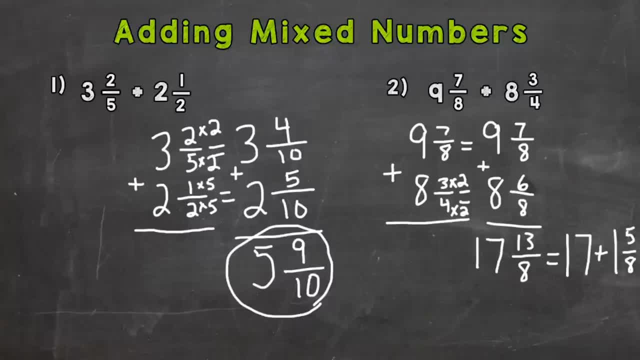 So we're going to get the denominator of 8 the same. So 13 eighths equals 1 eighths, 1 and 5 eighths. Well, we want to combine our whole numbers. That's 17 and that one whole. 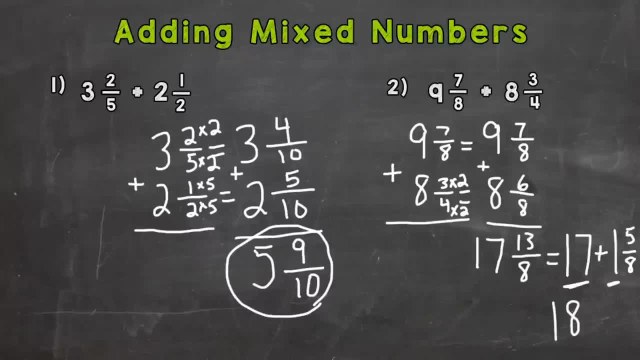 So our answer is actually going to have 18 wholes Plus- we don't want to forget about that- 5 eighths. So 18 and 5 eighths is our final answer for number 2.. So there you have it. 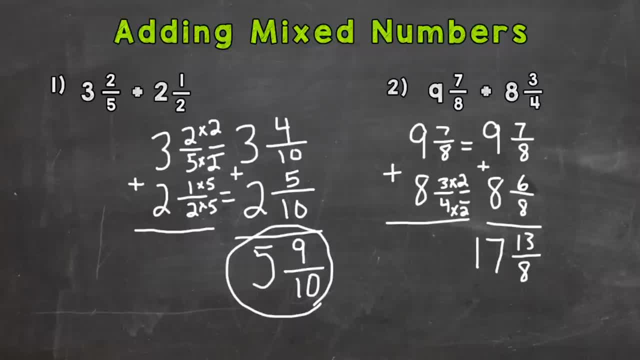 so we don't want to leave it like that. It's more than one whole, So we're going to change it to the mixed number and we need to combine the whole numbers together. So that's 17 plus whatever whole number we get out of that improper fraction. 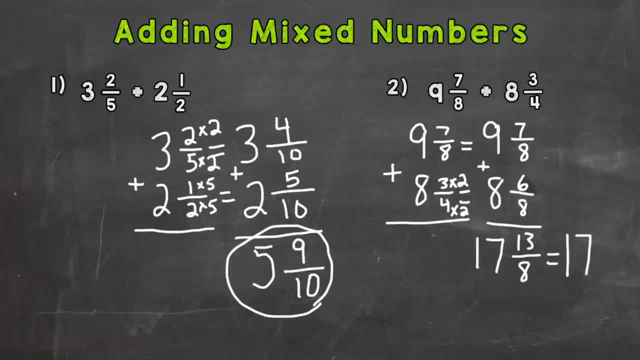 So we can think of it like this: 17 plus. well, to get improper to mixed number, we need to do: the top divided by the bottom, 13 divided by 8.. How many whole groups of 8 can we pull out of 13?? Well, one whole group with a remainder of 5.. 5 left over. Keep our 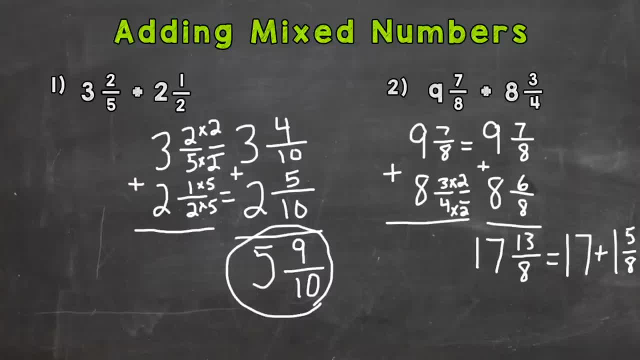 denominator of 8 the same. So 13 eighths equals 1 and 5 eighths. Well, we want to combine our whole numbers. That's 17 and that one whole. So our answer is actually going to have 18 wholes plus- we don't want to forget about that- 5 eighths. 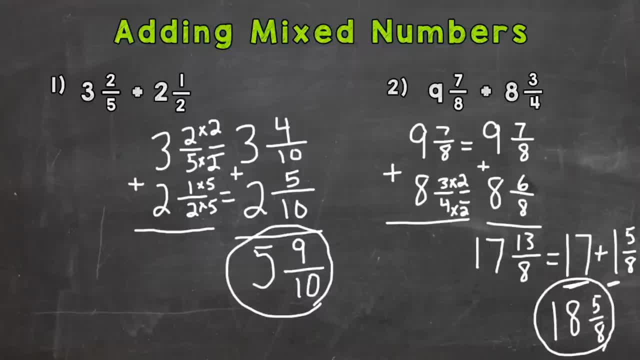 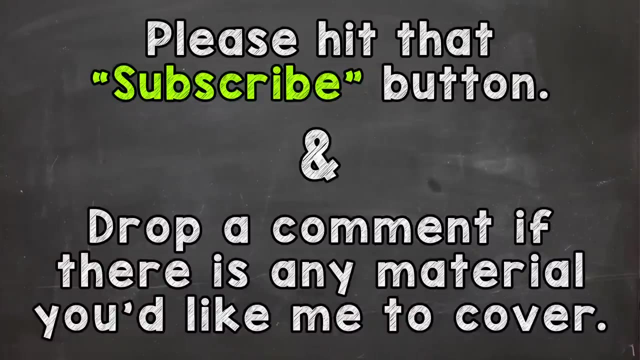 So 18 and 5 eighths is our final answer for number 2.. So there you have it. There's how you add mixed numbers. Hopefully that helped. Thanks so much for watching. Until next time, peace. 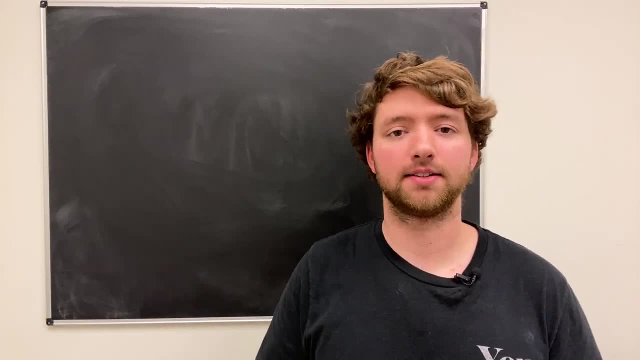 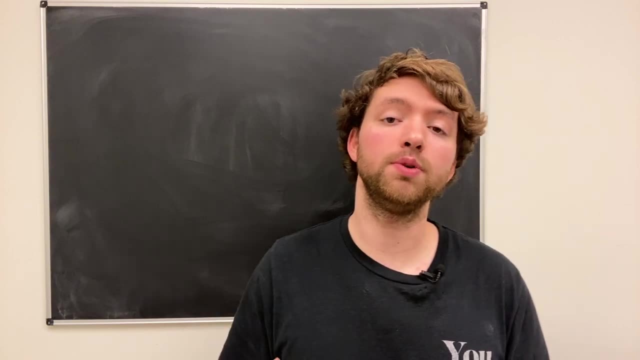 Hey, what's going on? everybody, In this episode we're going to be talking about linked lists. I did just do a video on arrays versus linked lists and some of the differences, but it was just an introduction, So if you want a little bit more substance, 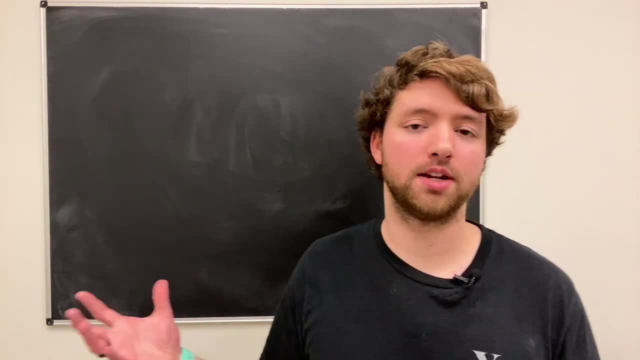 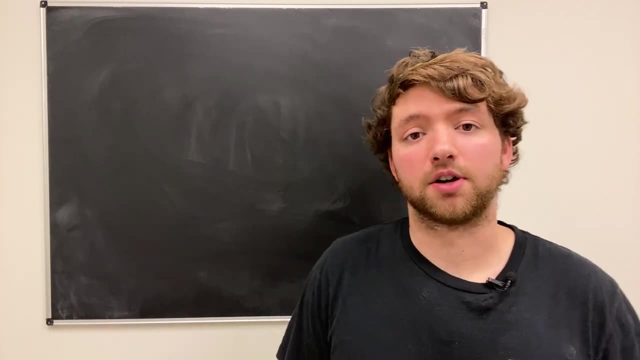 that's what this video is going to provide you, So hopefully by the end of this, you understand what a linked list is and some of the operations you can do on a linked list. So where do we even get started? A linked list is an example of a data structure. 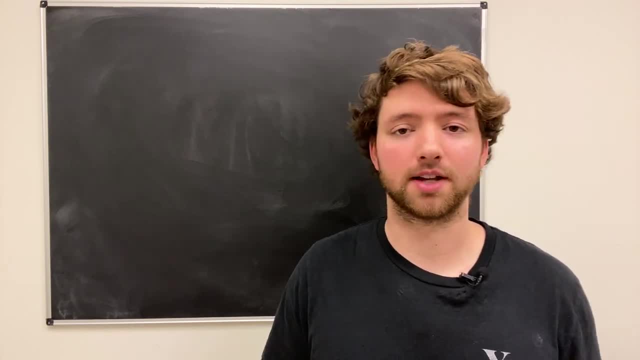 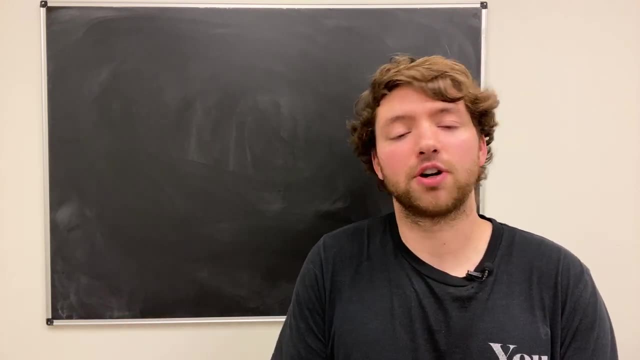 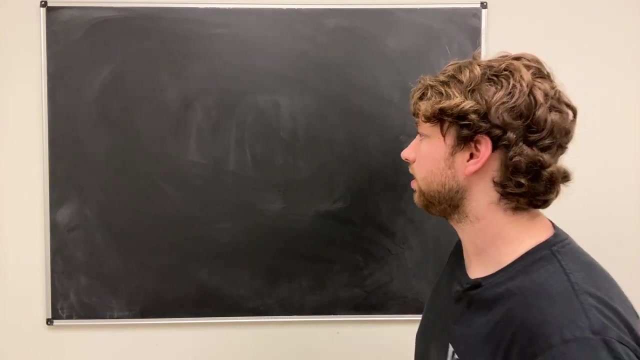 If you're in computer science, this word either excites you or makes you want to go cry yourself to sleep. Probably the second one there. but pretty much a data structure is just an arrangement of data. It's a way to store data. A very common one is a linked list. So with a linked list, 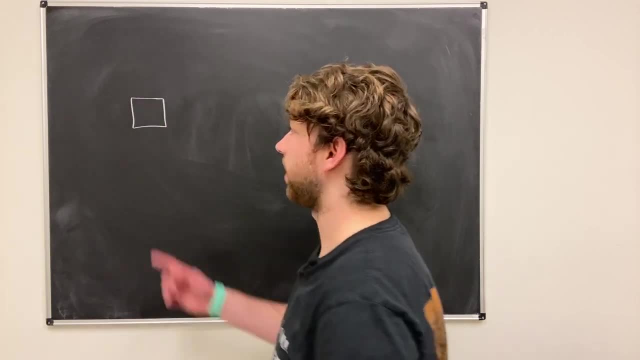 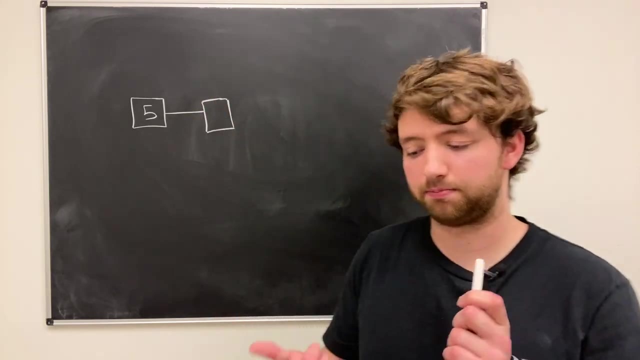 you can think of it as a chain where you have some data, and I'm just going to use numbers to begin with, but it could be anything. It could be a string, So it could be people's names, or it could be a string of numbers, So it could be a string of numbers, So it could be a string. 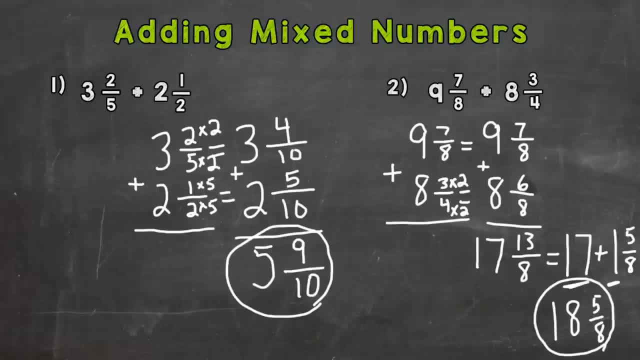 There's how you add mixed numbers. Hopefully that helped. Thanks so much for watching. Until next time, peace.